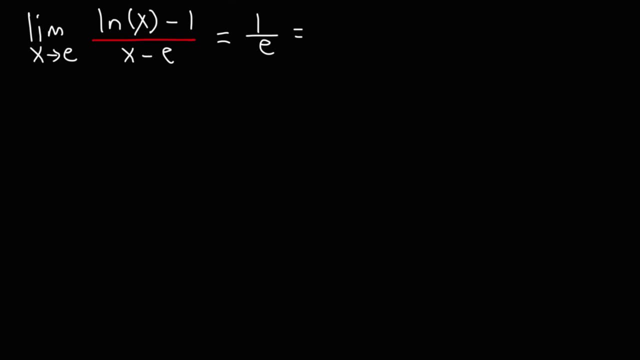 Let's get the decimal value of that: 1 over e is equal to 0.36.. So that's equal to 0.378794412.. Now e is a number as well. e is equal to 2.718281828.. 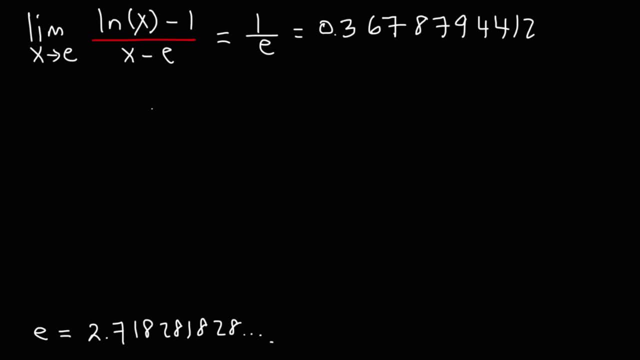 And the pattern continues. We're going to plug in an x value that is close to e, As x continues to approach e. if we get this number, then we know our answer is correct. So let's start. Let's start with 2.7.. 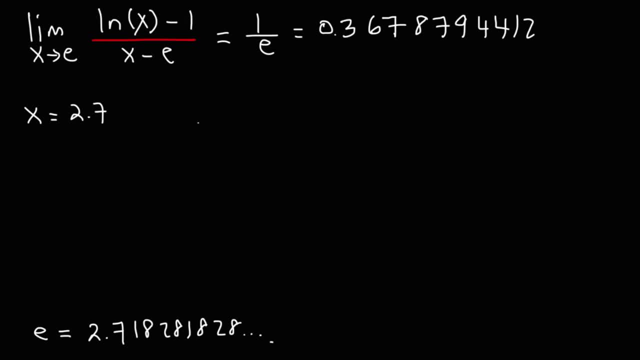 If x is 2.7, what is the value of that expression? So ln 2.7 minus 1 divided by 2.7 minus e, If you plug this in, you should get 0.3691221042.. 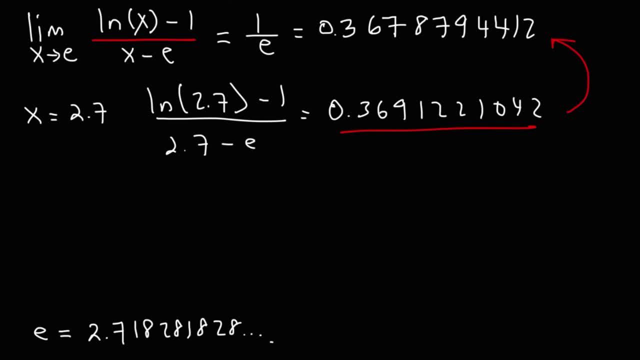 So it's not too far away from this value. But let's pick a number that's even closer. Let's try 2.718.. So if we plug in ln 2.718 minus 1 over 2.718 minus e. 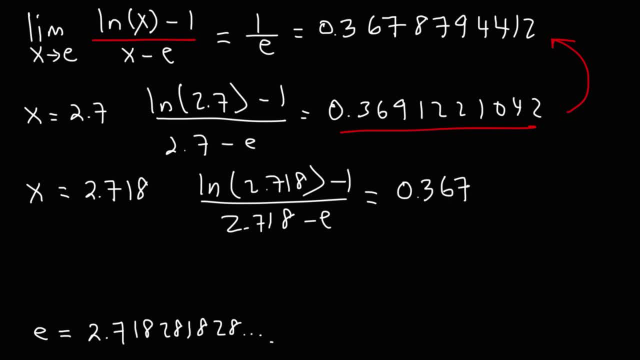 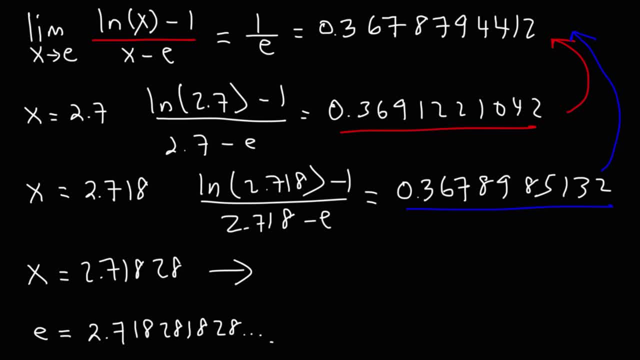 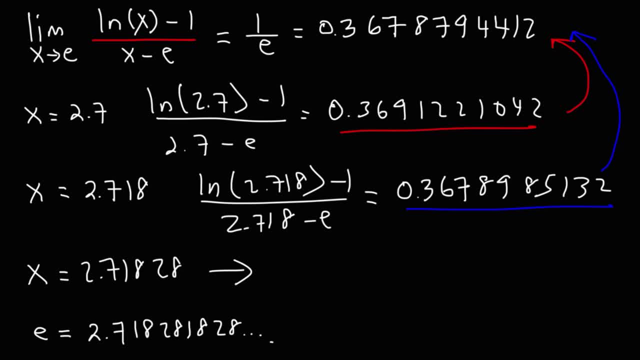